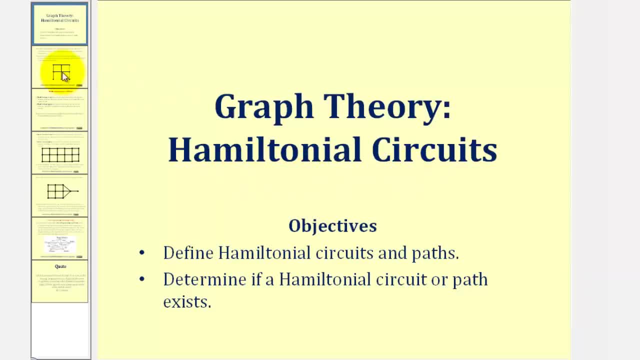 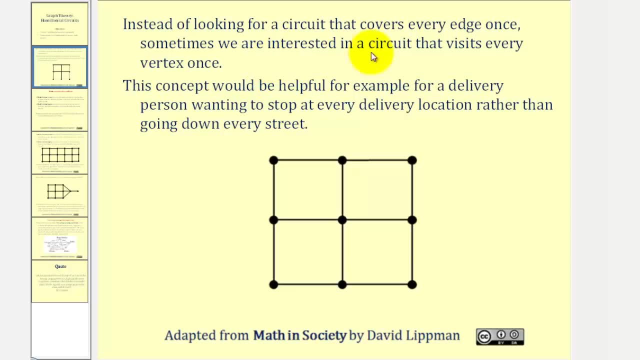 Welcome to a lesson on Hamiltonian circuits. Instead of looking for a circuit that covers every edge once, sometimes we're interested in a circuit that visits every vertex once. This concept would be helpful, for example, for a delivery person wanting to stop at every. 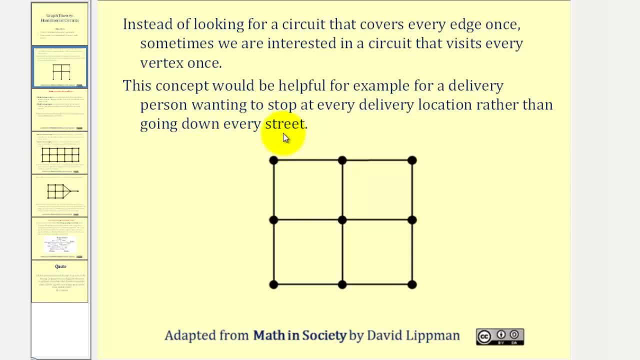 delivery location rather than going down every street. For example, if a delivery person needed to visit each vertex exactly once for deliveries, they might start here, go in this direction, turn. go in this direction, turn and then go in this direction. 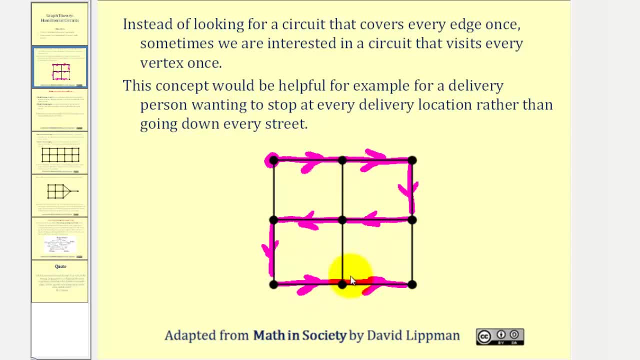 Notice how this would be a path rather than a circuit, because the starting vertex and ending vertex are not the same, And notice how the delivery person could also take different routes and still visit each vertex exactly once. For example, the delivery person again might start here. 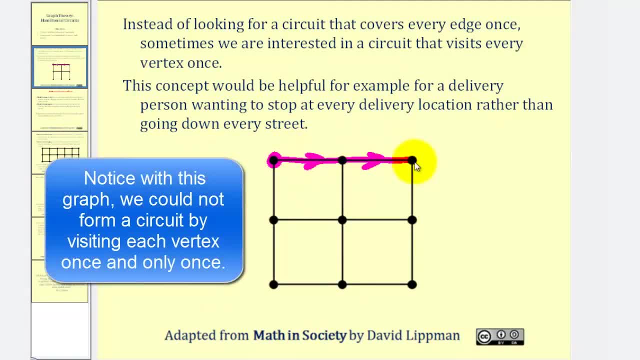 go in this direction, turn and go in this direction, turn and go in this direction, turn and go in this direction and turn again here. So the delivery person would start here and end here, and again notice how this is not a circuit. 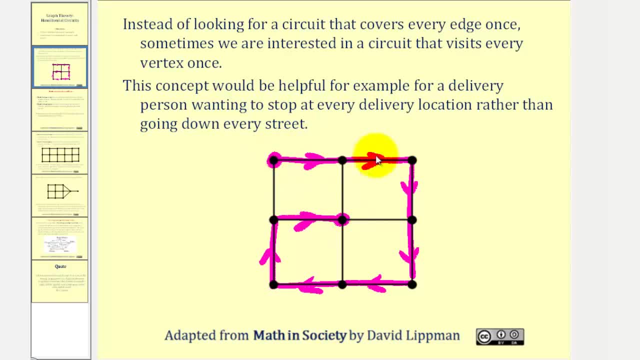 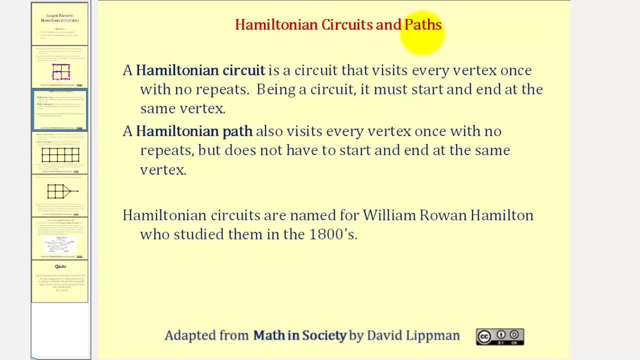 it is a path, but it does visit each vertex exactly one time, Which leads us to the definitions of Hamiltonian circuits and Hamiltonian paths. A Hamiltonian circuit is a circuit that visits every vertex once, with no repeats. Being a circuit, it must start and end at the same vertex. 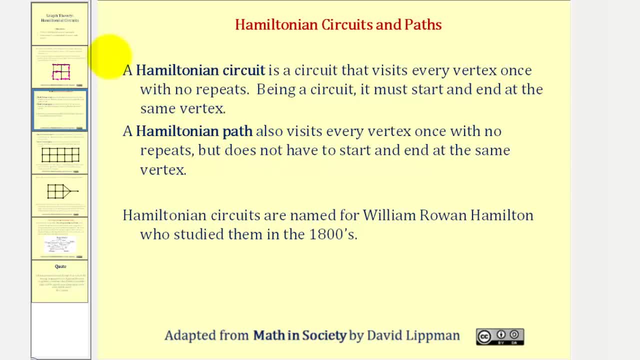 A Hamiltonian path, which we saw in our previous example, also visits every vertex once, but it does not visit every vertex once with no repeats, but does not have to start and end at the same vertex And Hamiltonian circuits are named after. 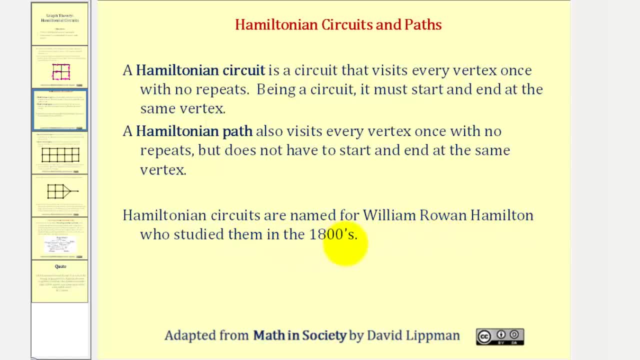 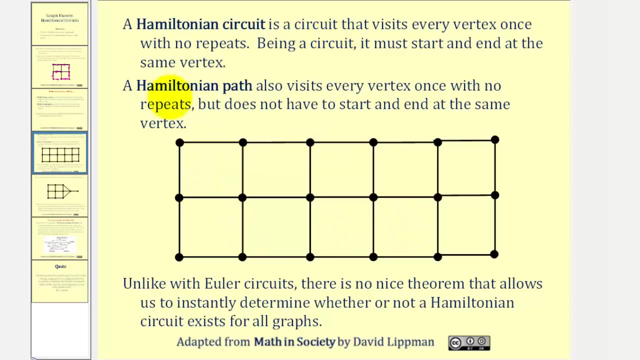 William Rowan Hamilton, who studied them in the eighteen hundreds. Let's take a look at a couple more examples. Let's take a look at another example. Let's see if we can find a Hamiltonian circuit for this graph here, Which means, if we start here. 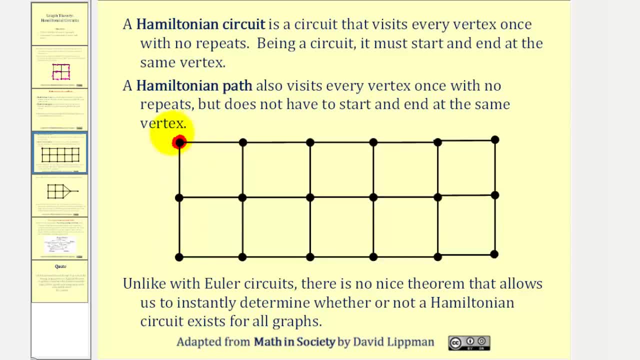 we want to visit each vertex exactly one time And return to this vertex, So we can start in this direction, Turn, turn, turn and keep this pattern going, Turn and go all the way to here And return to the starting vertex. 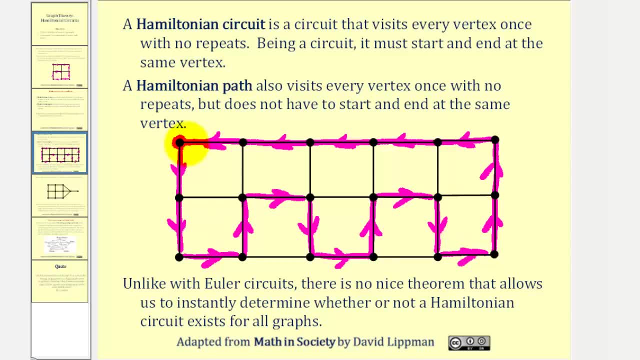 This is an example of a Hamiltonian circuit. We started here, visited each vertex exactly one time and ended back at the same vertex. A Hamiltonian path also visits every vertex once, with no repeats, but does not have to start and end at the same vertex. 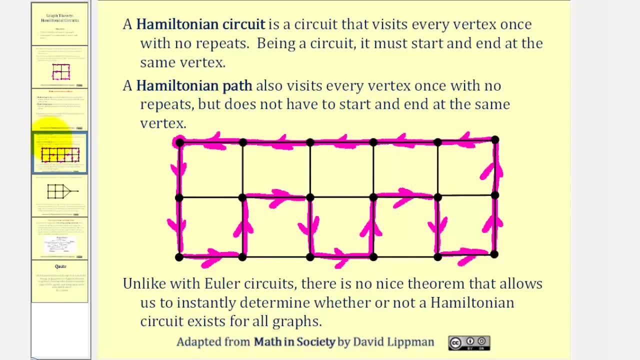 And we saw a couple of these using our delivery person example. Let's see if we can find a Hamiltonian path for this graph. So we'll clear the Hamiltonian circuit, So we'll start here again And notice how we can go in this direction all the way to the end. 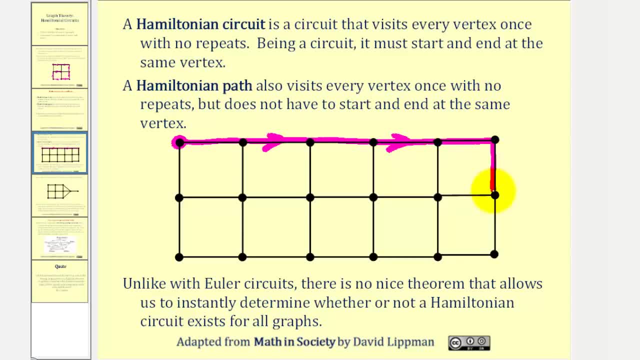 Turn, Go all the way back in this direction, Turn Then go back in this direction, And this is how we started here: Visited each vertex exactly one time and ended here in a different location. This is an example of a Hamiltonian path. 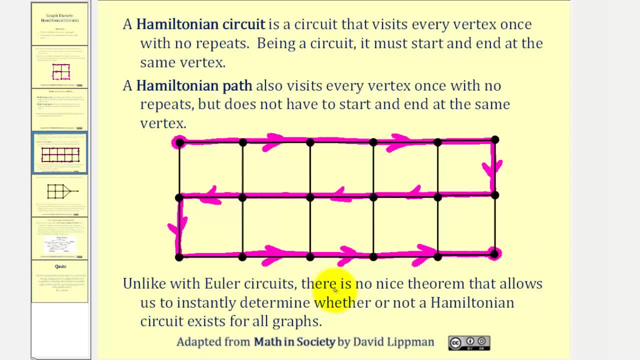 Now it's important to recognize that, unlike Euler circuits, there is no nice theorem that allows us to instantly determine whether or not a Hamiltonian circuit exists For all graphs. Let's take a look at another example. We want to determine if a Hamiltonian path or circuit exists. 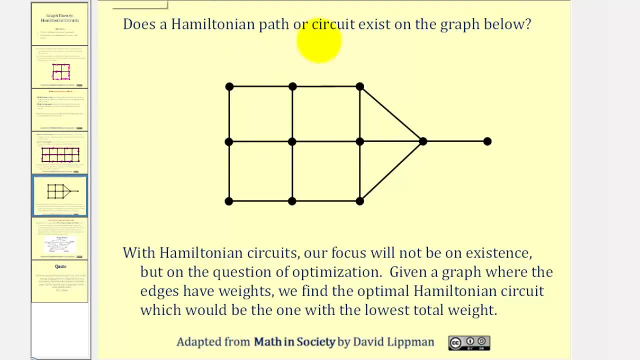 on the graph below. Let's first consider a Hamiltonian circuit. Looking at the graph, notice how, if we were to start at this vertex here, there's no way that we could visit each vertex exactly one time and return back to this vertex because of this single edge here. 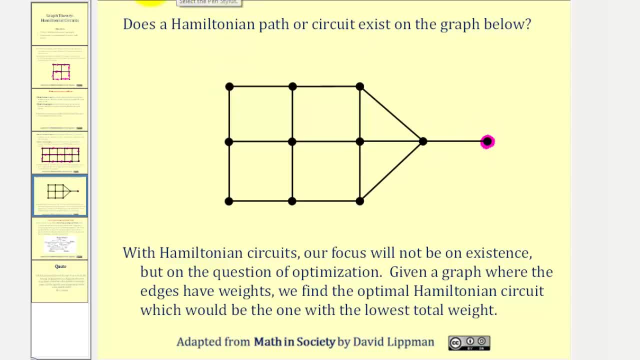 So a Hamiltonian circuit does not exist. Let's see if we can find a Hamiltonian path, meaning we can start here, visit each vertex exactly one time, but we don't have to end back at this vertex. So we could go in this direction. 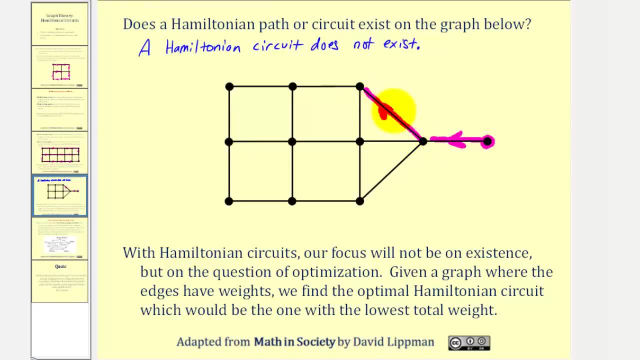 Maybe turn in this direction, Turn and go in this direction, Turn and go in this direction, Turn, Turn And turn. This would be a possible Hamiltonian path. Notice how we visited each vertex exactly one time, with no repeats, and therefore this is a possible Hamiltonian path. 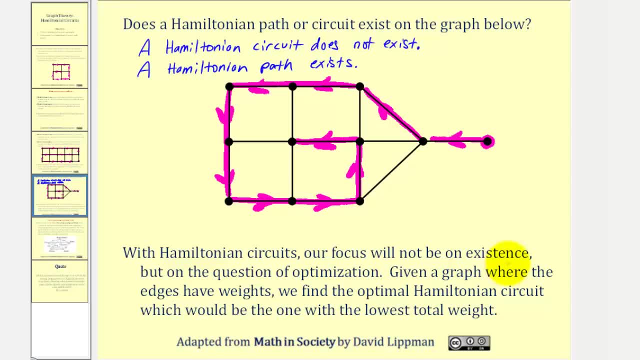 With Hamiltonian circuits, our focus will not be on existence, but on the question of optimization. Given a graph where the edges have weights, we want to find the optimal Hamiltonian circuit, which should be the one with the lowest total weight, Which brings us to a famous problem. 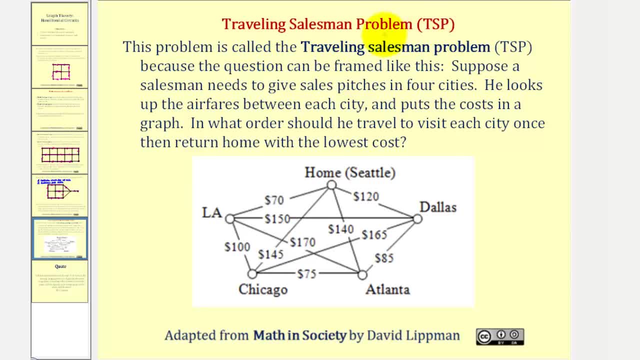 called the traveling salesman problem, or TSP for short. This problem is called the traveling salesman problem because the question can be framed like this: Suppose a salesperson needs to give sales pitches in four cities different from their home city. He looks up the airfares between each city. 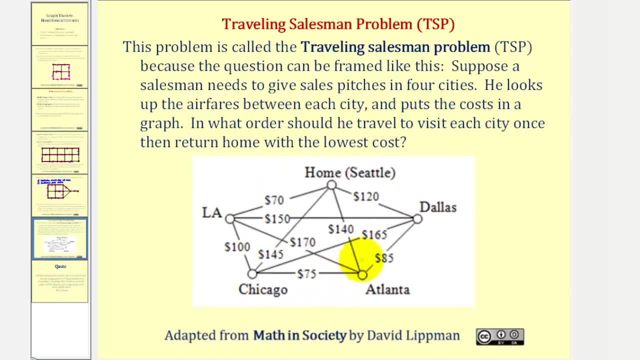 and puts the cost in a graph, as we see here below. In what order should he travel to visit each city once, then return home with the lowest cost? Let's look at one possible Hamiltonian circuit. If the salesman starts here in Seattle. 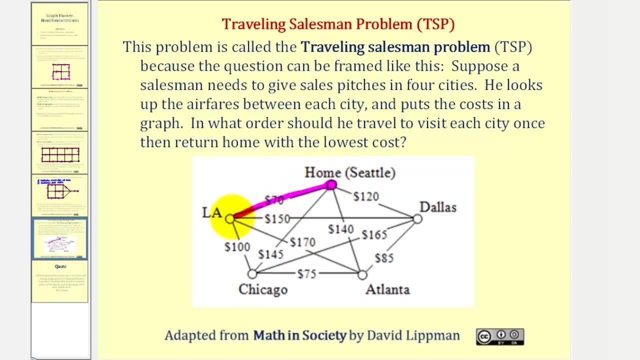 let's say, maybe they fly to LA, which would cost $70.. And then from LA, let's say, to Chicago for $100., Maybe to Dallas for $165, then to Atlanta and finally back home to Seattle, Notice using this Hamiltonian circuit.